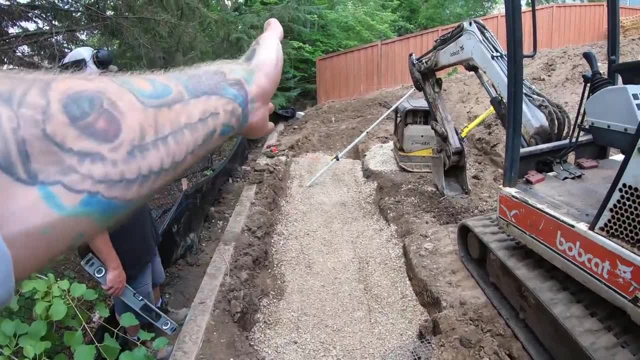 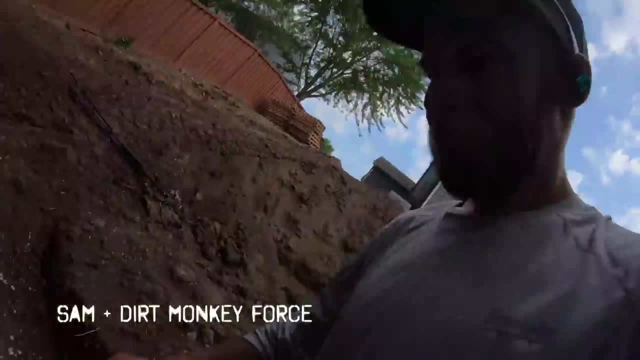 just gonna lay out a couple timbers holding the base blocks. It's not gonna fly For a massive nine foot wall that's going to be holding back an entire yard. But once we get these timbers out of here then we can kind of see if we want to do a step down in this area or if we can get our three. 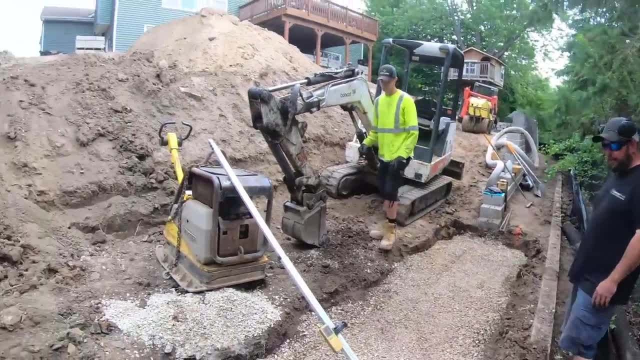 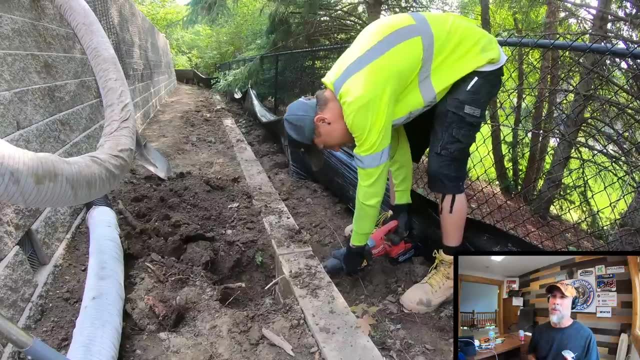 to one slope, but these timbers need to be gone regardless. All right, I got the saws all up there for you, bud. All right, let's pop them. All right. so let's talk about what we're doing at the base: a really steep slope, and we're gonna be building a retaining wall on that steep. 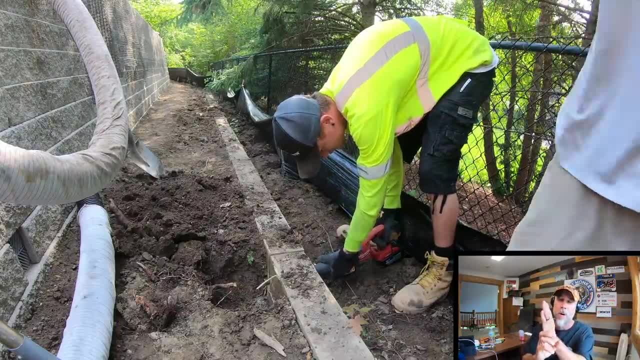 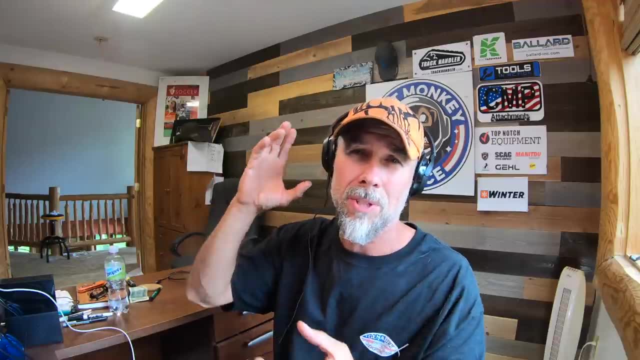 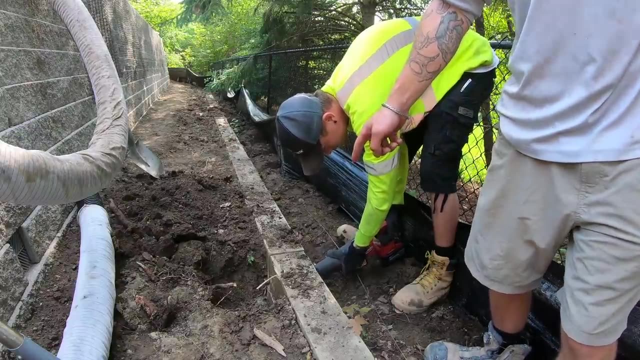 slope. we've got to embed more of the retaining wall, meaning we've got to get more of the blocks buried. so in this case, Tim wanted those timbers removed so that he could actually bury more of the base block. he got it right at the scene. so actually, yeah, yeah here, look out of the ways he's gonna pull a stop one off. 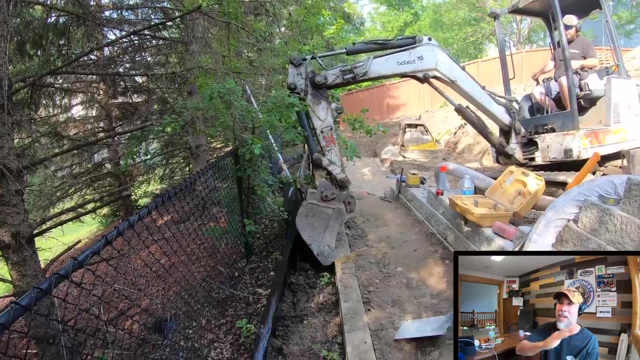 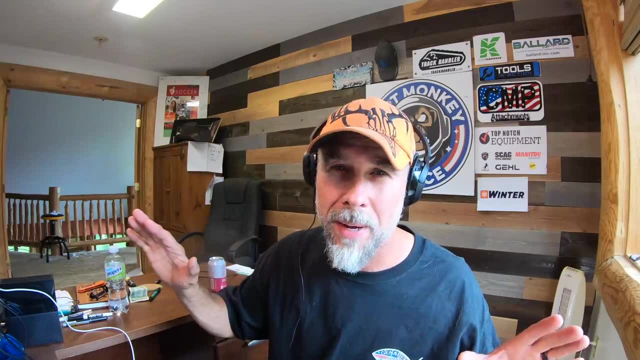 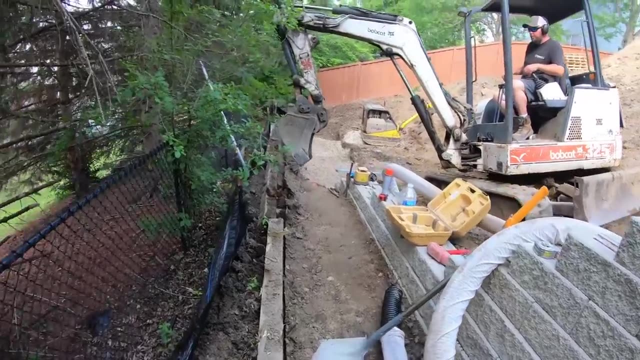 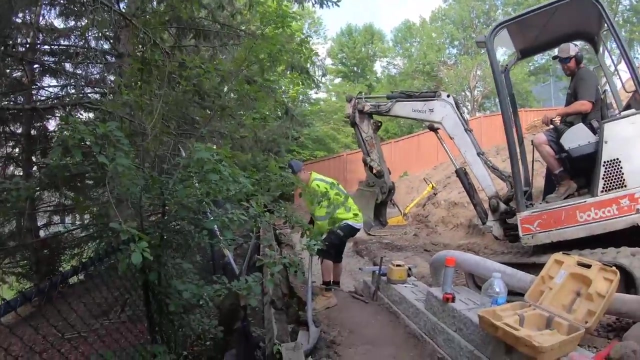 for you. if he left those in place and those fell away, we may have one or two courses of block that should be buried exposed. the wall wouldn't fail by any means. he's just going above and above, over and above. Get it around the joint there. He's got some monster. he put some monster lay bolts in it. 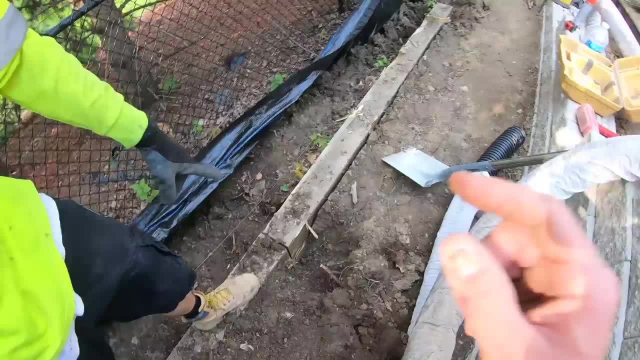 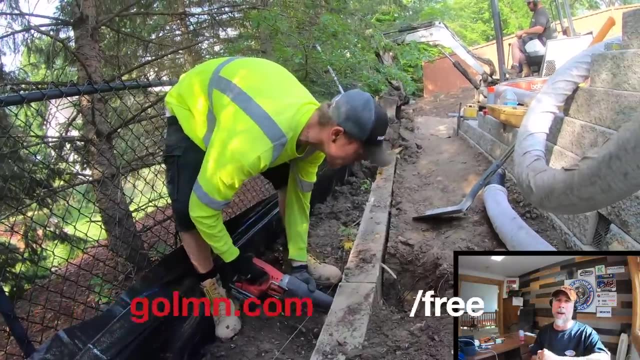 here, so you don't even need to get through all the way on that bottom one. if you just get through most of the way he can, he can snap it, and today's video is brought to you by our friends from LMN software. these guys helped me be. 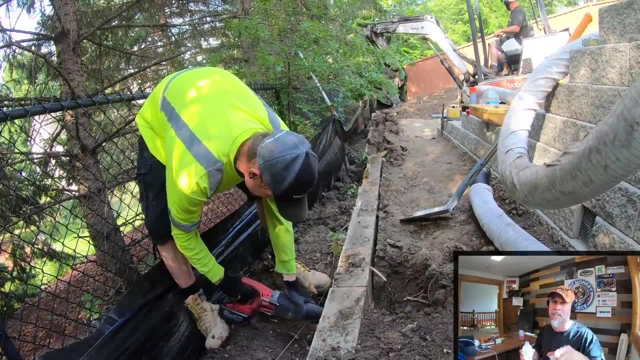 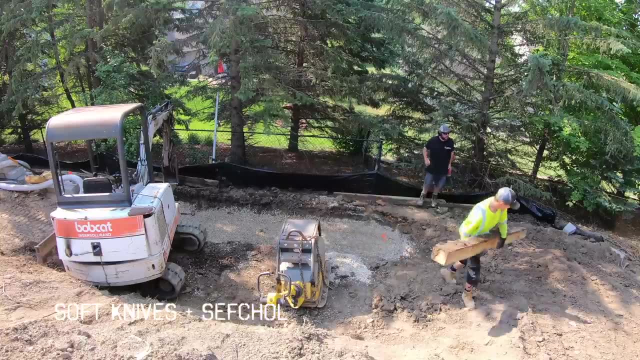 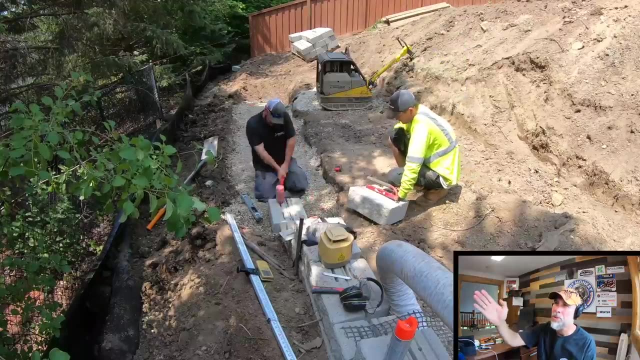 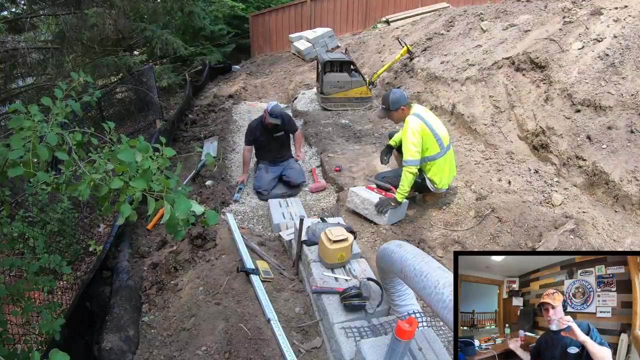 able to free up my time to make videos that help you guys out. what Tim is doing right here is he's actually basing a step up, and so to base a step up, this is where, instead of stepping the slope down, we're stepping it up. we actually put one block on top of another block, so we have two. 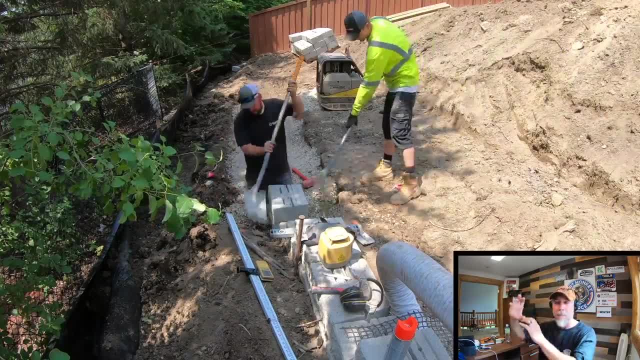 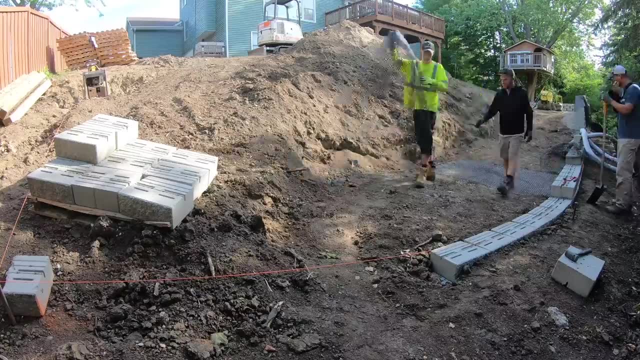 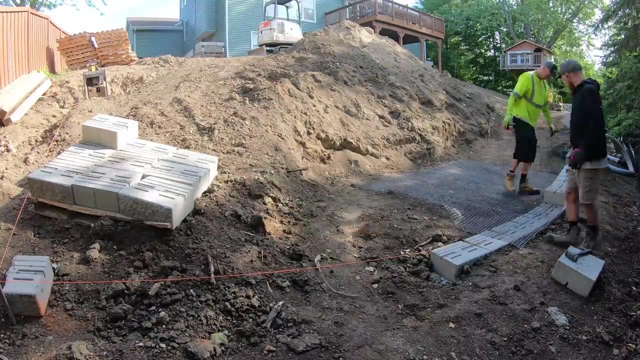 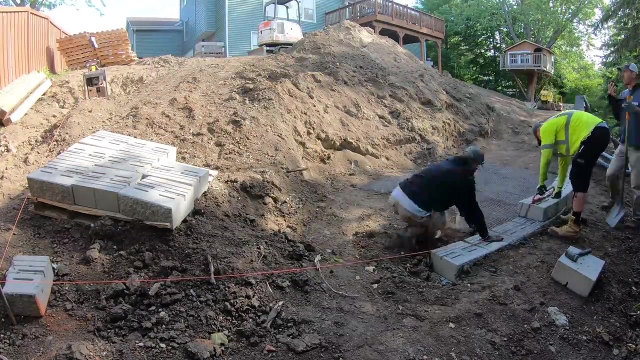 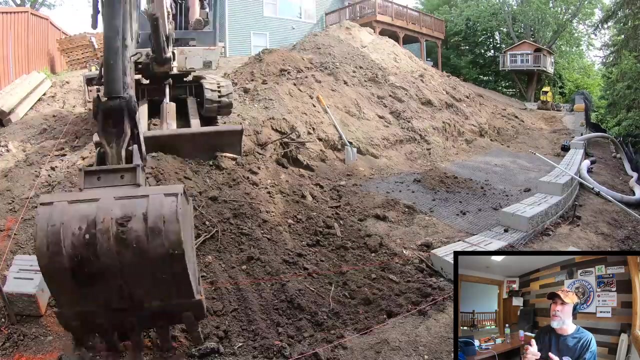 blocks equal to each other, and what that does is that allows us to keep all of our courses aligned. now, when you're building an engineered retaining wall, one of the most critical things that you've got a nail is the geo grid and the geo grid, if you look right. 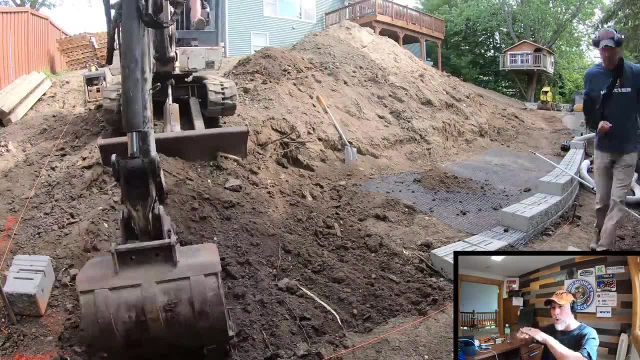 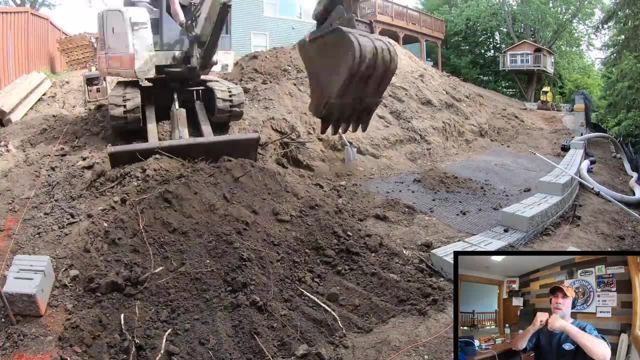 here is that black mesh like fabric that lays horizontally behind the retaining wall. that geo grid locks into the face of the wall. and when you're building an engineered retaining wall, that geo grid locks into the face of the retaining wall and what it does is it holds the face of the retaining wall with all of the soil behind it. so 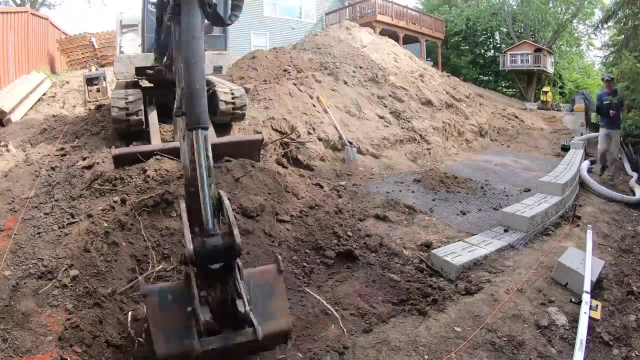 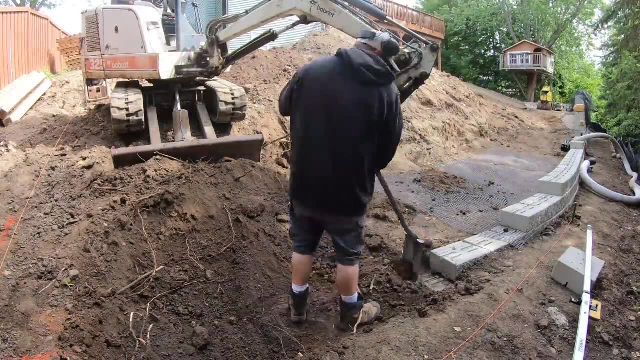 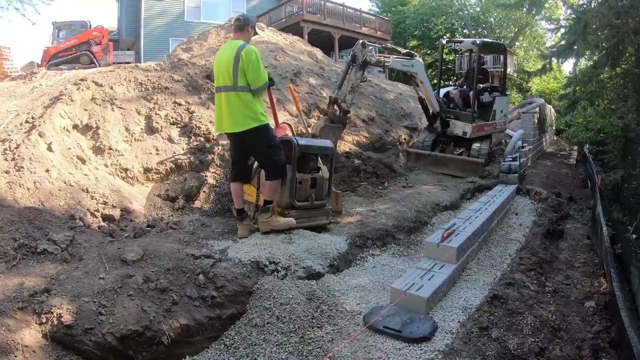 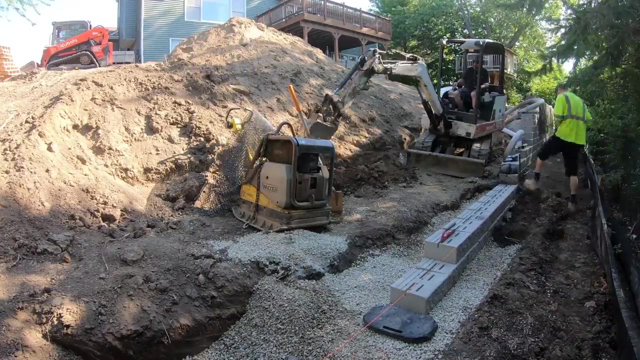 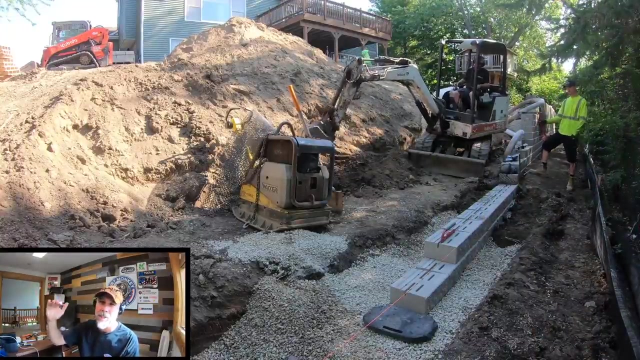 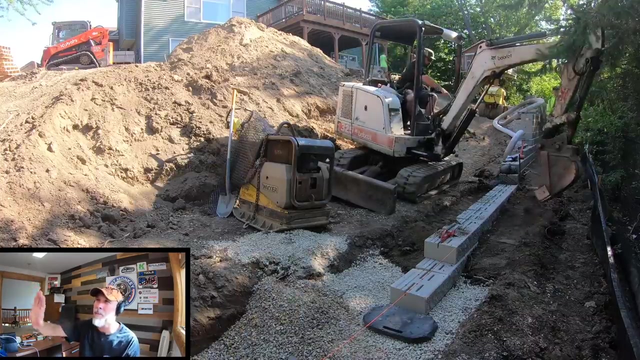 that everything then moves as one mass. so if you look a little further down the wall right here, you can see that on this slope we're burying three courses. two courses are getting buried right here, but further down the line you can see where an actual third course is buried. 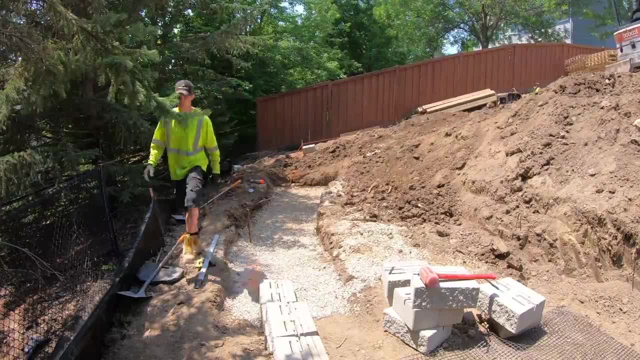 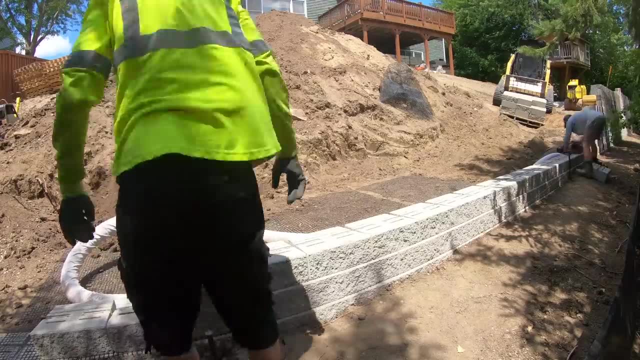 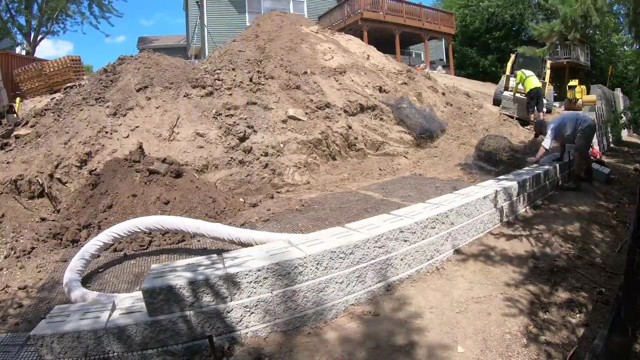 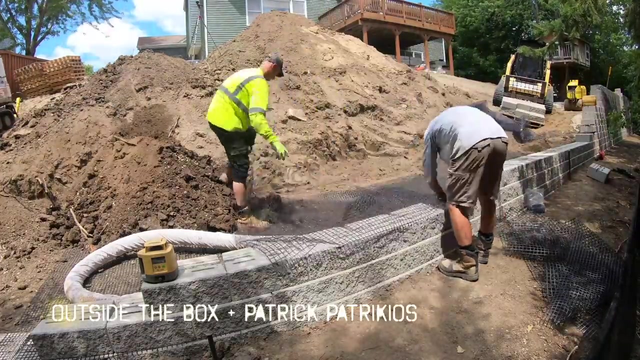 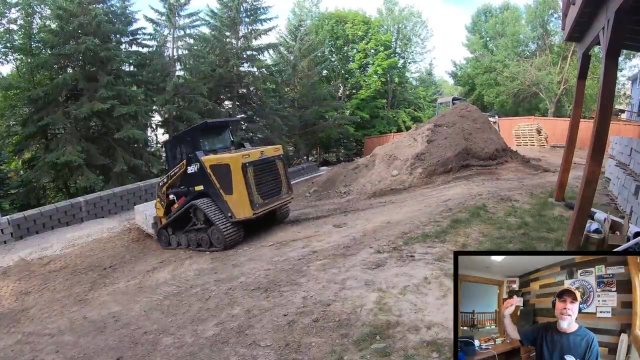 letting everything come together, so you're gonna have to deal with building 14gr. where are we on this slope 14gr now? so let me go over here and let you take a look, so So if you look, you'll see us dry stacking the wall and we can actually dry stack the. 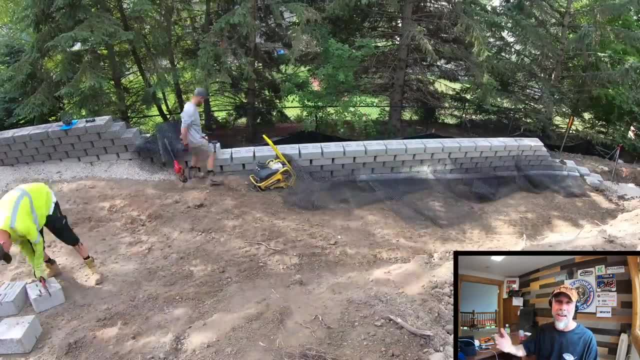 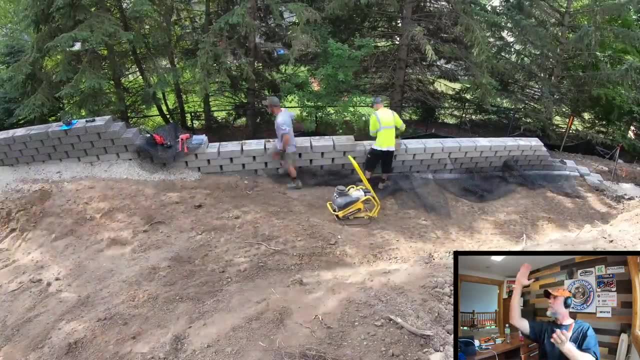 wall about four courses before we're forced to backfill it. And what we do is we can flip, we put the grid down and then we stack, stack, stack, and then we flip the grid up. we pack, pack, pack, put the grid down at the appropriate. 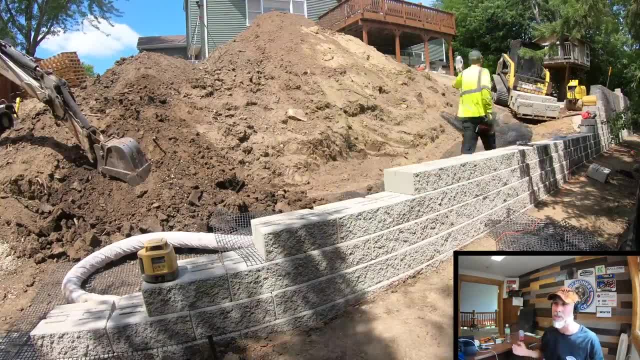 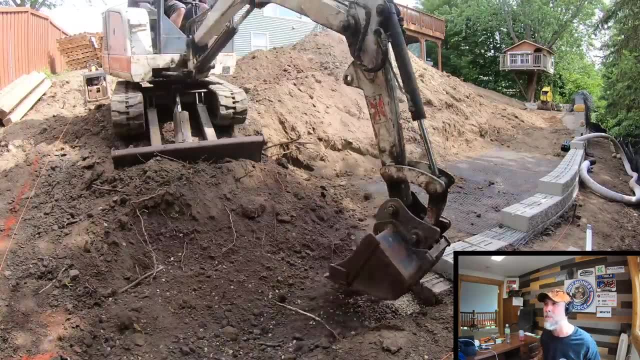 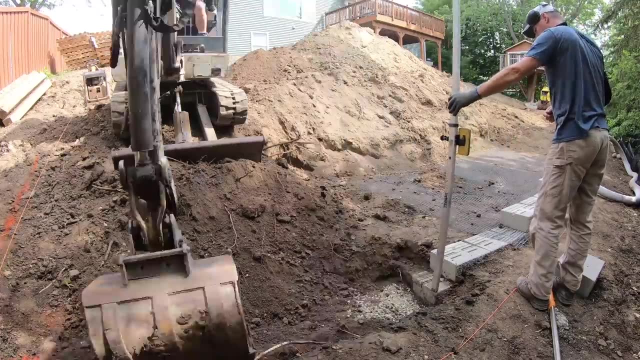 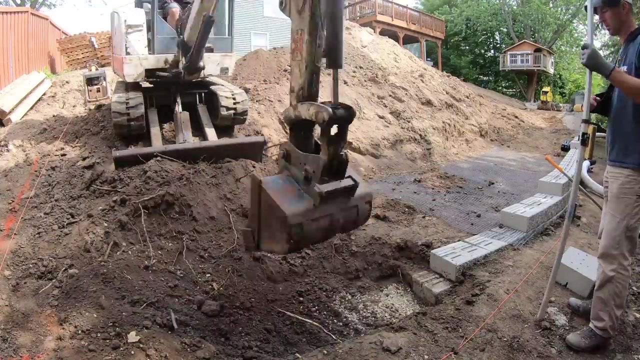 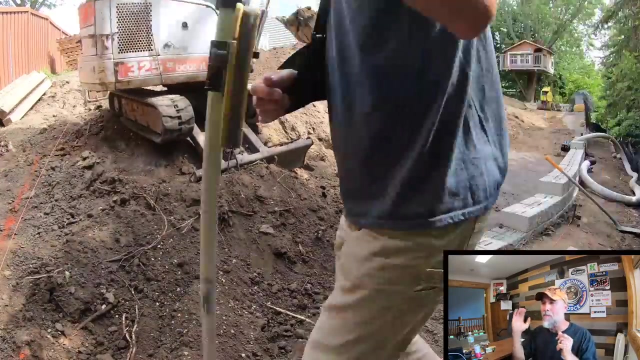 level, then continue to pack until we get to our four courses before we wash, rinse and repeat that same process over again. That's a little trick we use to speed up the process. So here's kind of a fun fact. You'll see that we're installing drain tile into the retaining wall. but if you ever drive, 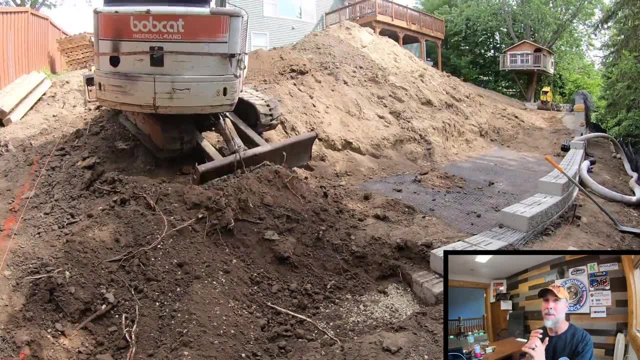 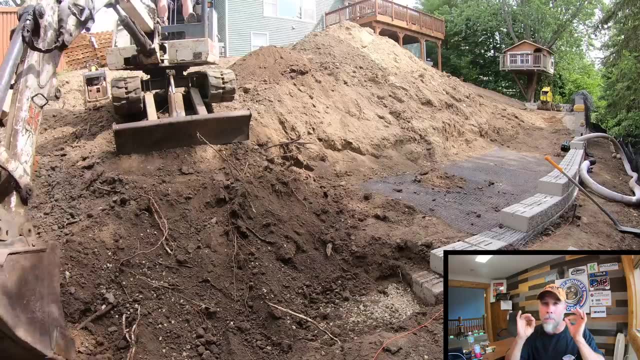 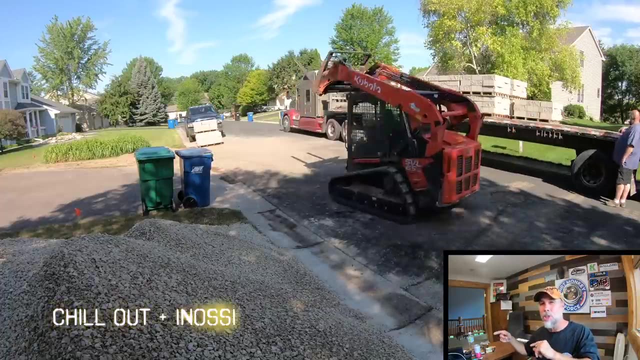 by a retaining wall and you see the drain tile actually operating. it means that that wall is in a state of failure. Okay, They see, on modular retaining walls like this, they are a mortar list system intentionally and we use a lot of drainage aggregate and you're going to see that in just a moment. 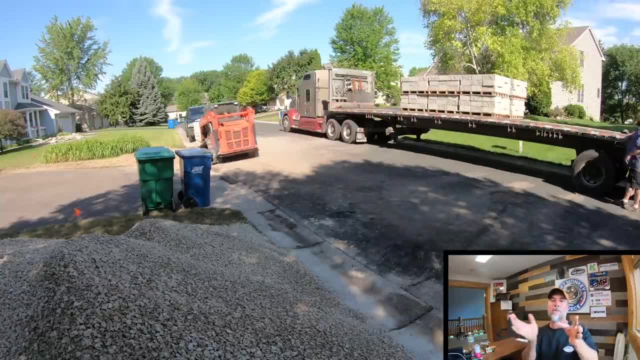 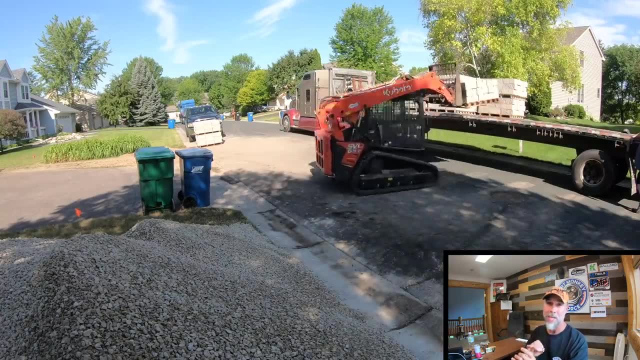 but the entire retaining wall is designed to allow water to flow freely right through the face of it. So if you ever actually see the water being funneled or jetted out through the drain tile at the bottom, it means whatever company installed that retaining wall didn't put enough drainage. 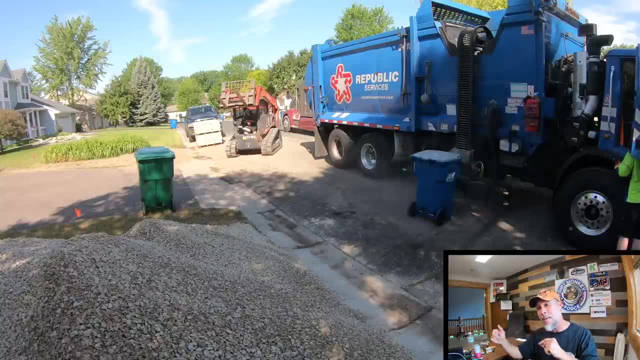 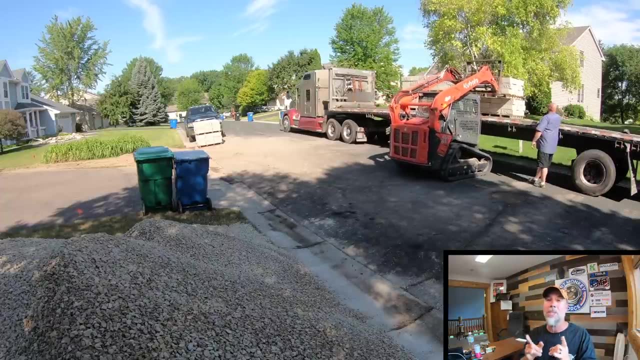 aggregate in, Or that That drainage aggregate that may be in place is boogered up and not operating. So either way, if you've seen drain tile operating in a modular retaining wall, something is wrong. That's a big red flag. 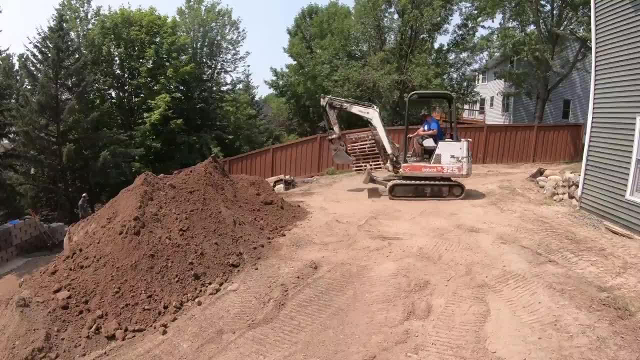 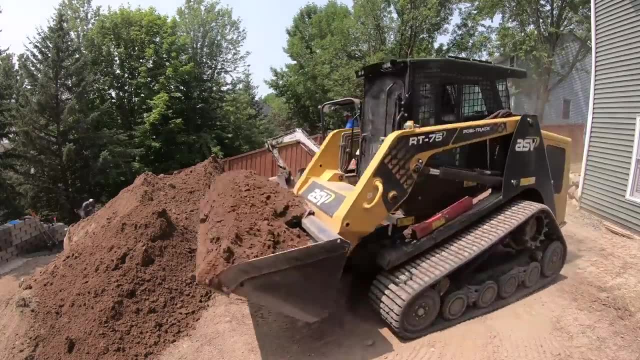 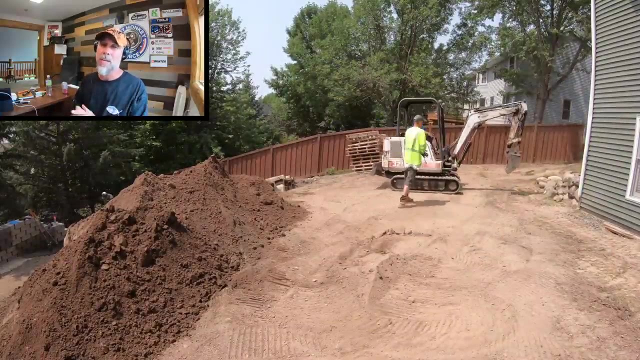 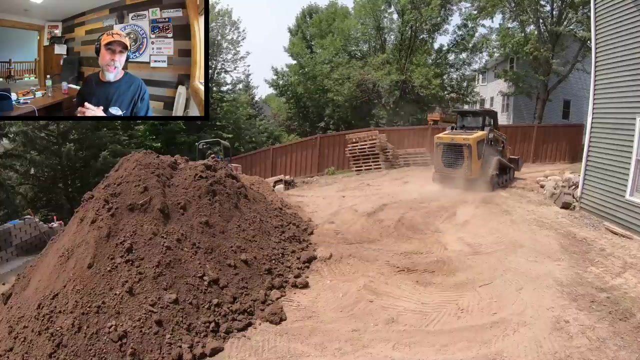 So we're going to show you what it looks like. So, on this project, we ended up bringing in about 45 dump truck loads of structural fill soil, And instead of showing you each and every load going in, we just thought we'd show you. 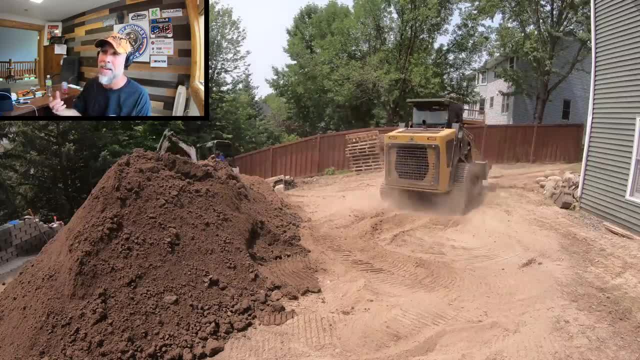 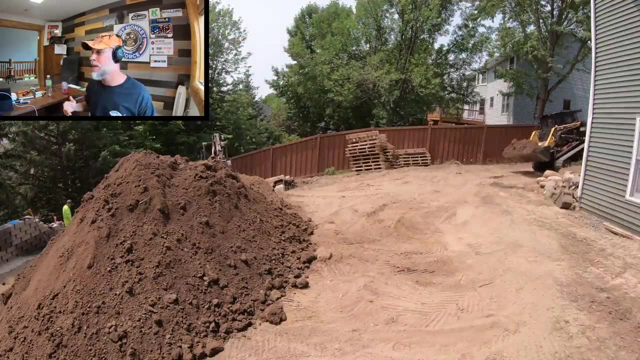 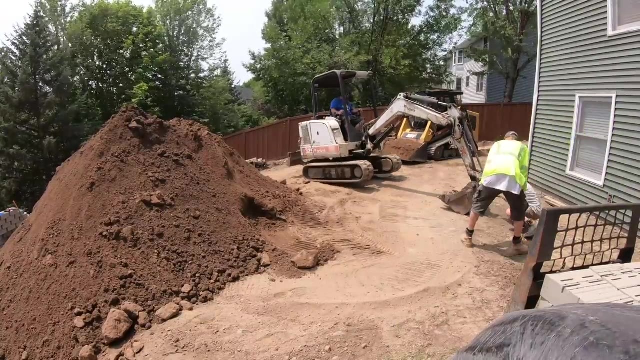 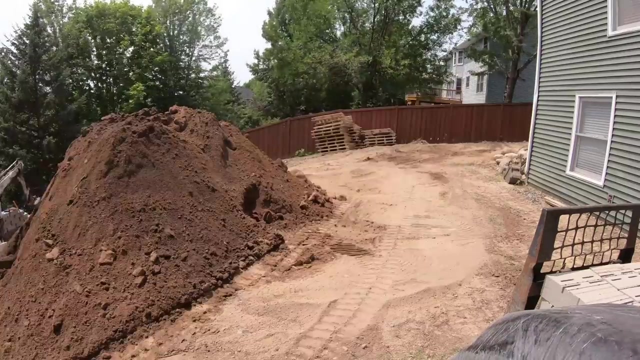 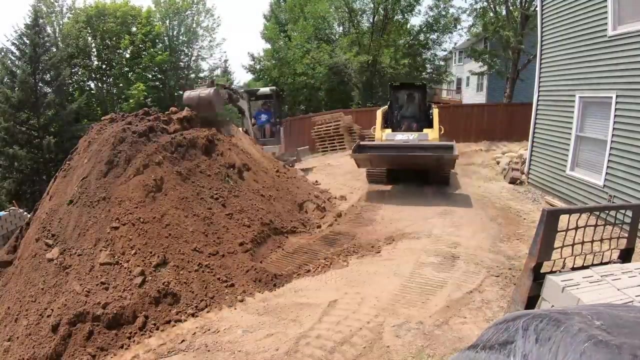 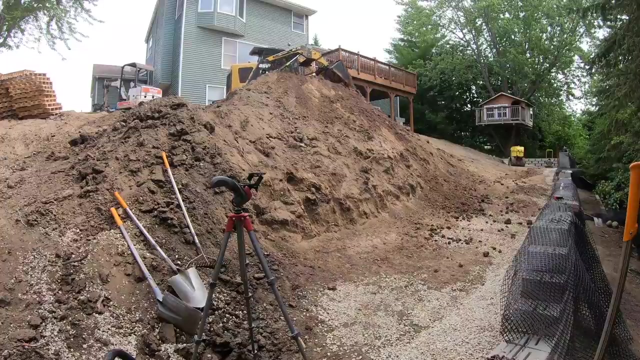 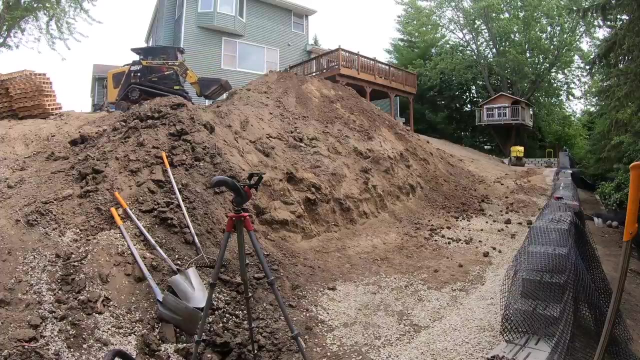 what it looked like So you could get a gist of what we're using. Okay, So what we're using- and that is a granular material with a clay binder in it which allows us to pack it up tight like concrete- Yeah, so now, now he's got to get in there and mix it all together so that we can get. 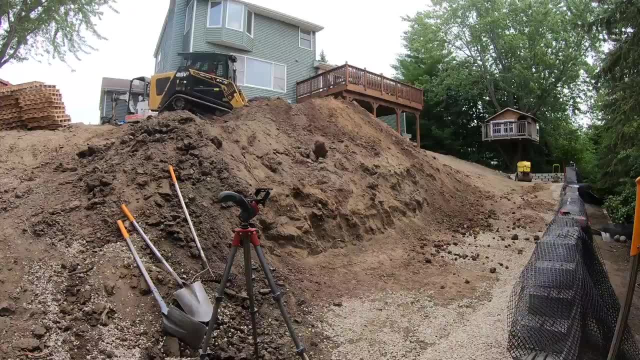 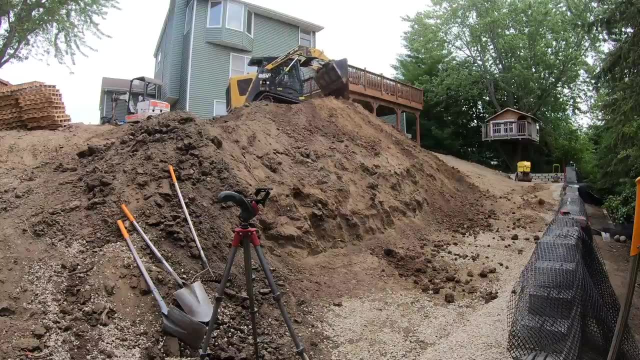 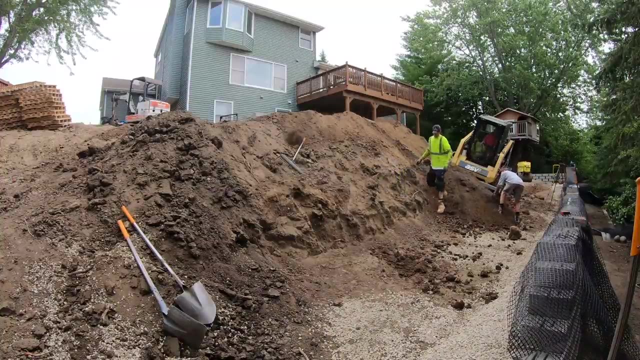 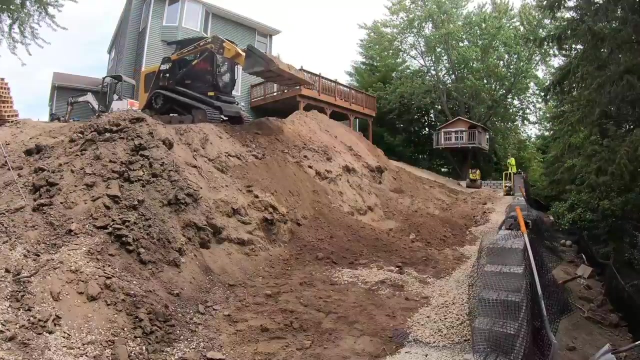 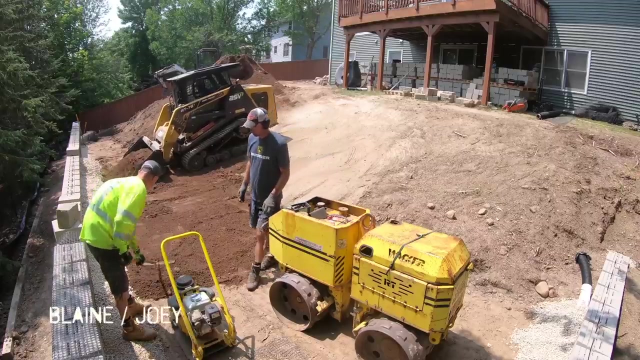 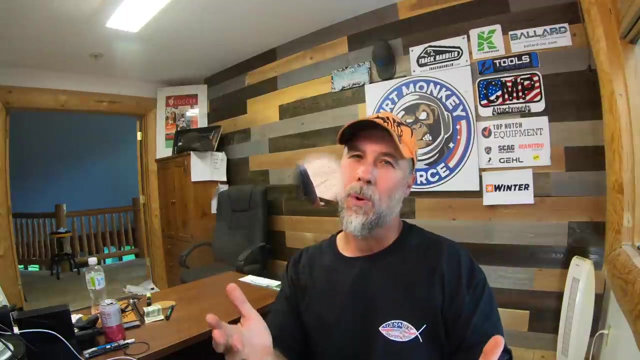 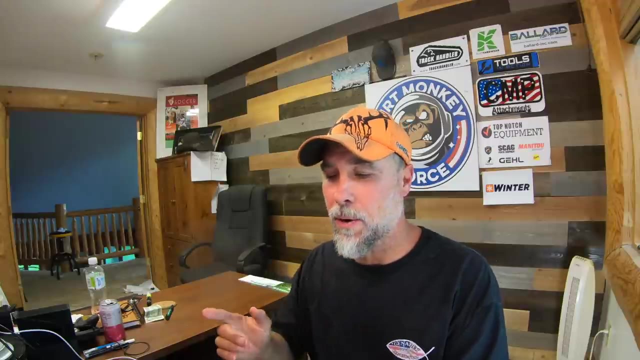 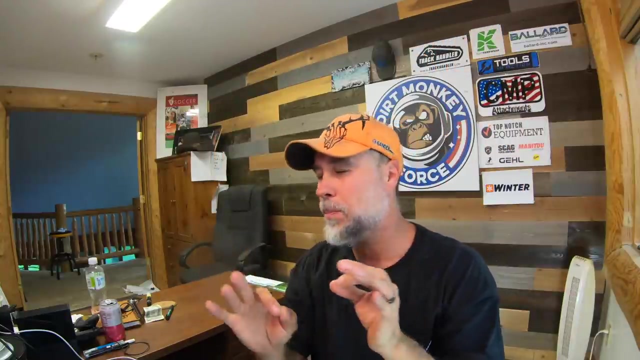 it to pack, Oh that back up into there. So more than one of you guys have asked me, Stan, what do you think of the ASV versus the CAT, versus the Kubota? And here's the breakdown: We love the cab on the Kubota hands down, love that swing up door, but the CAT has buttery. 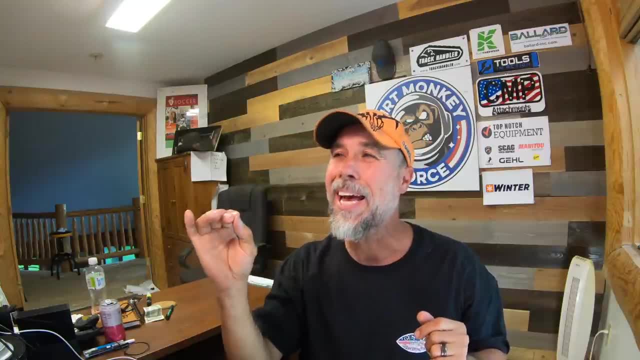 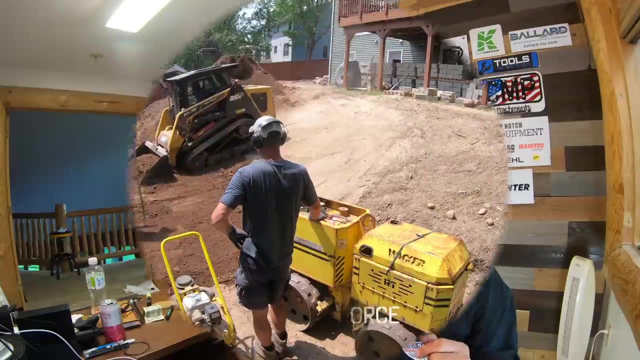 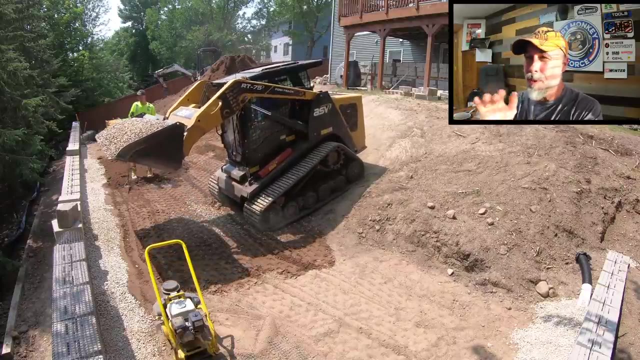 smooth controls, but the ASV, when it comes to just sketchy slopes, that's the machine that the guys go to, So that, right, there is a really sketchy move. There's zero tolerance. When a skid loader is going to fall over, it'll tip over sideways, but it'll also likely. 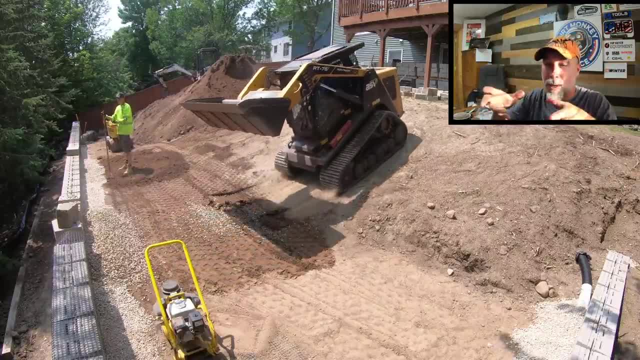 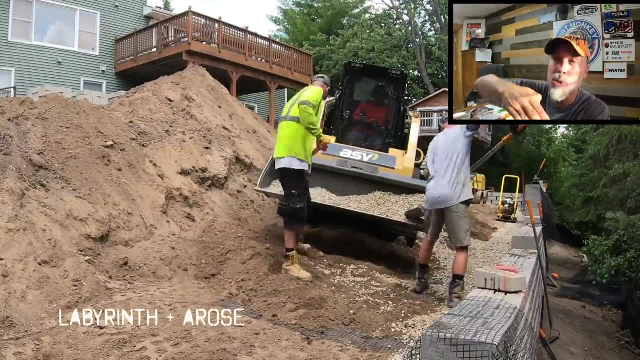 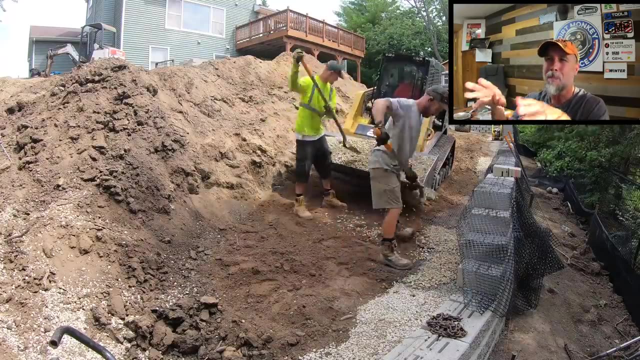 tip forward And as he's coming down the slope, especially with weight in the bucket, all of the weight of that machine is now transferring forward, And when you're driving down to a retaining wall, if that machine decides to go forward, typically you can just catch yourself with your bucket. 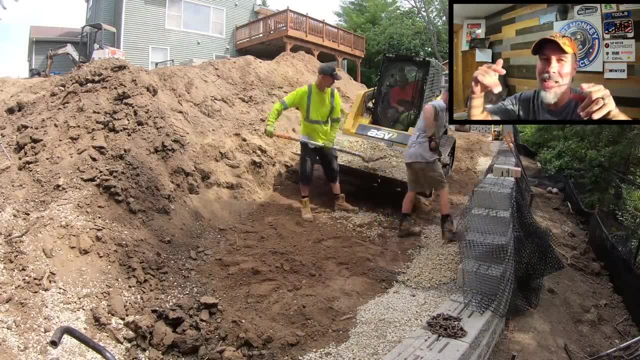 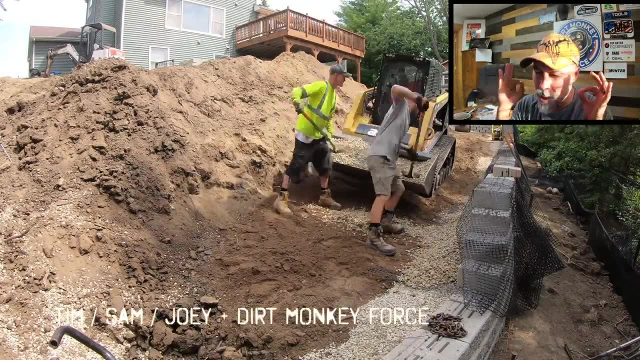 But when you have a retaining wall and you're coming right up to the edge of it a lot of times, if your machine falls forward, the bucket will fall over the face of the retaining wall, putting the operator in a really jeopardizing situation. 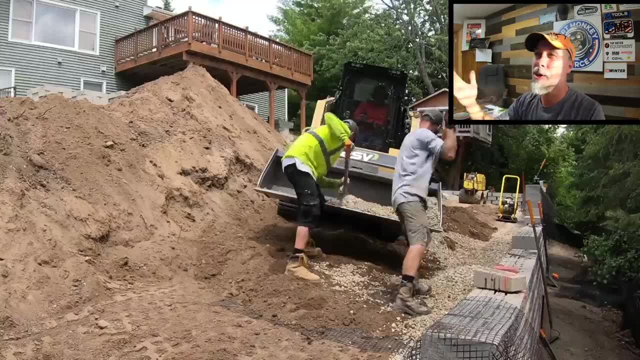 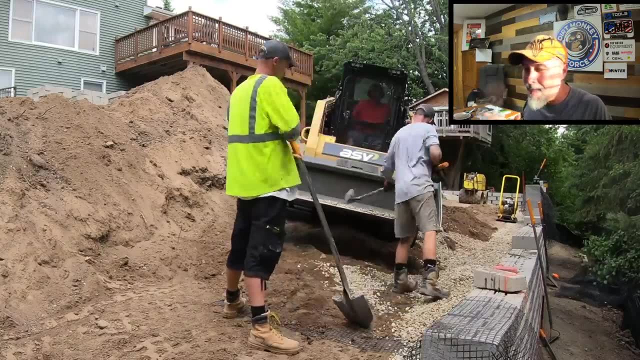 So although it doesn't look like much on film, a good operator knows that that right there is a sketchy place to be, And these guys have learned to trust on that ASV. They've gotten that machine dialed in And they know exactly what to do. 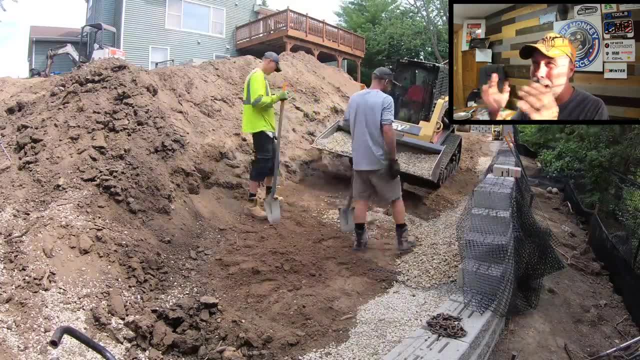 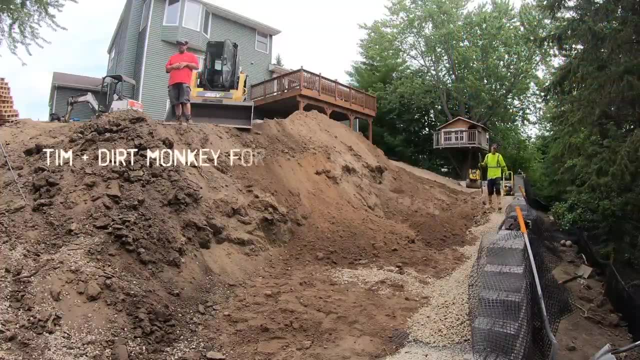 Exactly where its capabilities are. So, when it comes to sketchy slopes, that's why these guys migrate to this machine. We're going to use up probably all this dirt today. huh Yeah, that's good. I'd like to save some for this over the weekend. 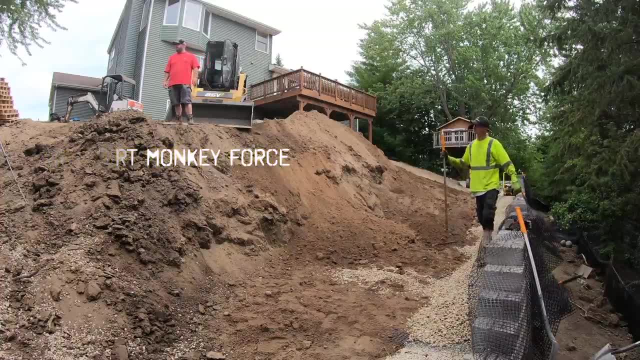 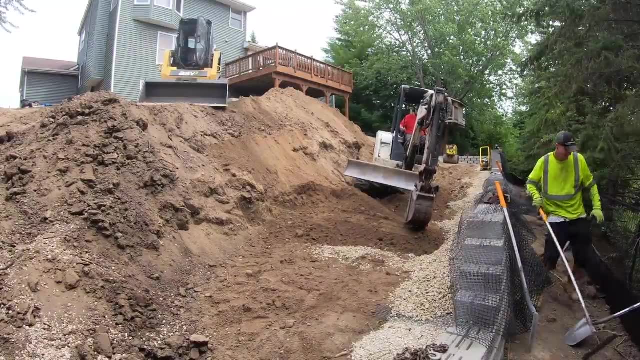 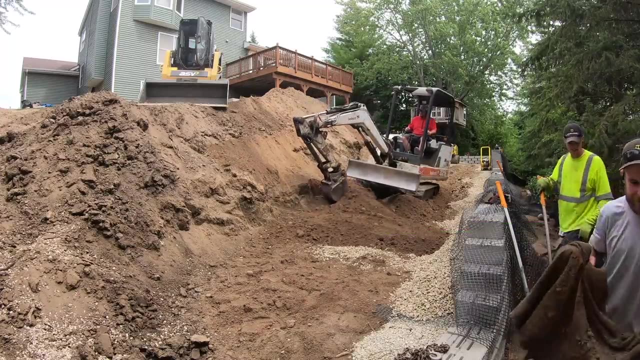 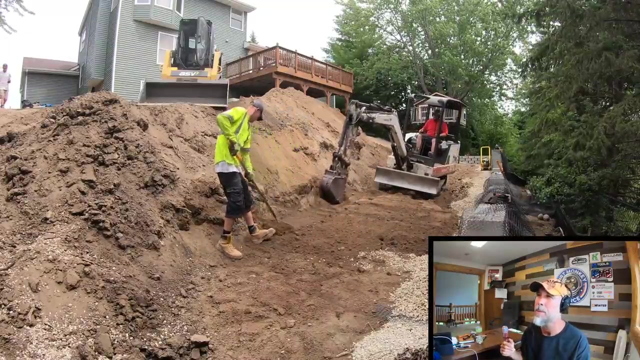 We've got to be able to backfill this all up and protect it. if I get something in, Yep, Something's got to get in. though Where did that come from Carpet? Yeah, I don't know. So what they're doing right here is prepping a geogrid zone. 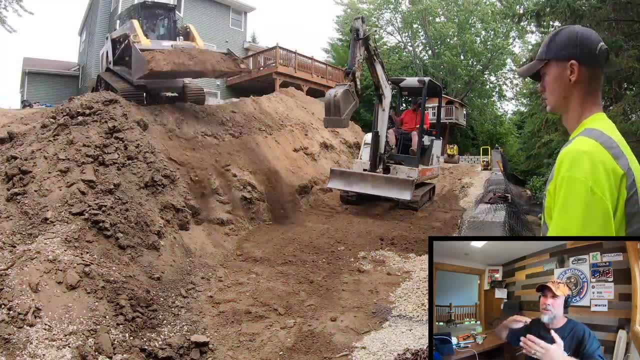 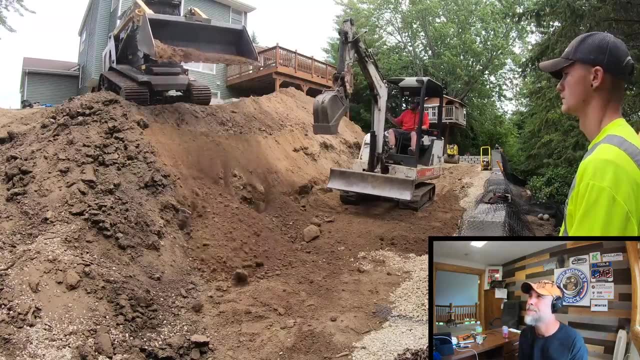 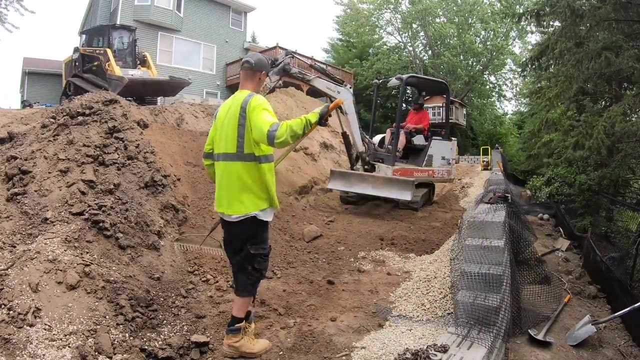 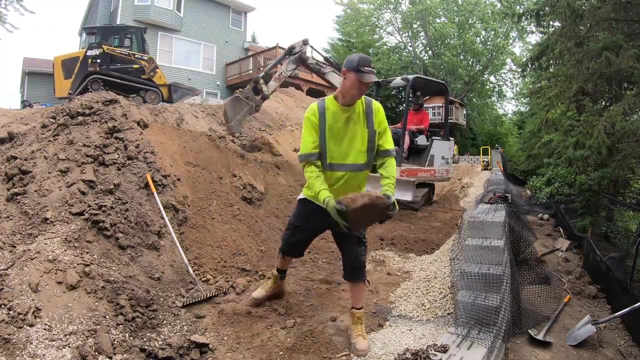 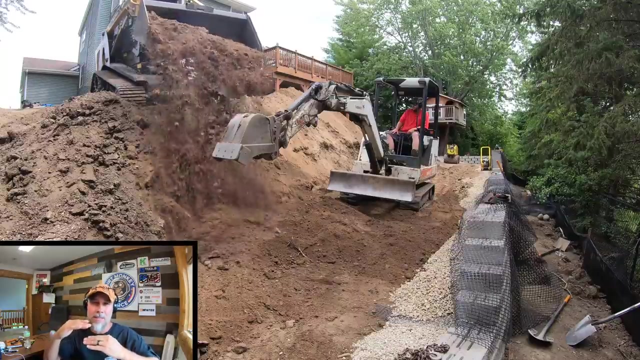 And prepping a geogrid zone means they're going to flatten it out so that they can pack it, so that they can fold the geogrid down and then put more dirt over the top of it. We go with very thin lifts because this allows us to see what material is actually. 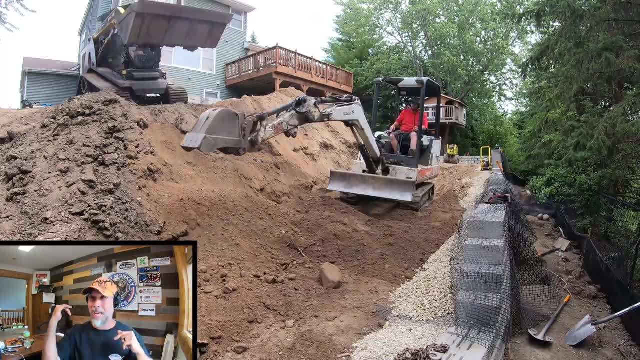 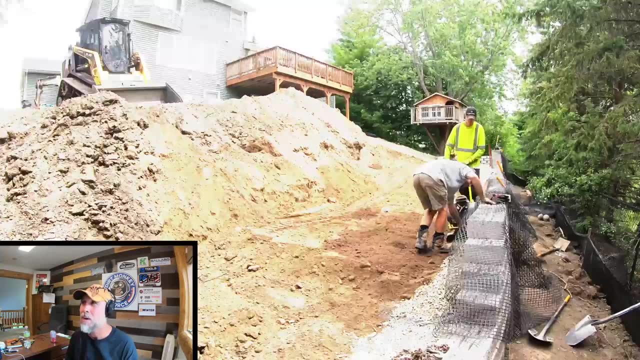 going in place. Big rocks aren't allowed. Things like whatever that was we found earlier is not allowed. Roots get pulled out, Anything that doesn't look structural gets yanked, And then, as we get real close to the wall, we have to fix it. 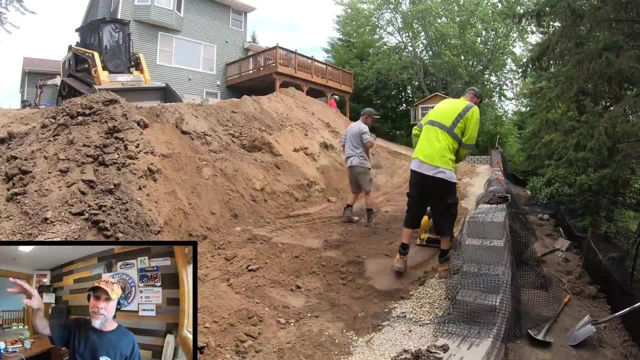 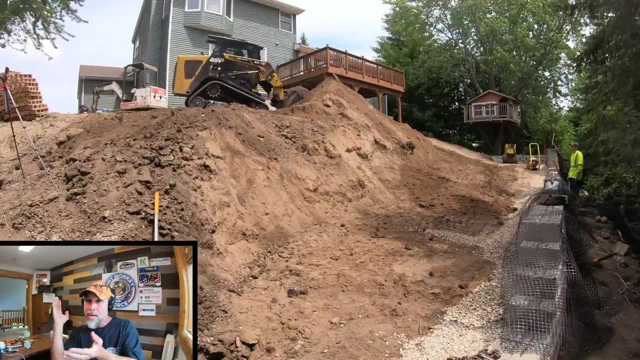 Yeah, we use two different compactors. In the draining zone you'll see that we're using the 150 pound plate packer because it's not gonna shift the wall out, And then in the reinforcement zone we switch over and we use our big packer. 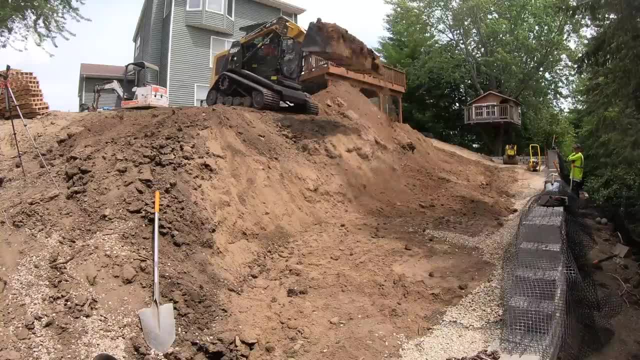 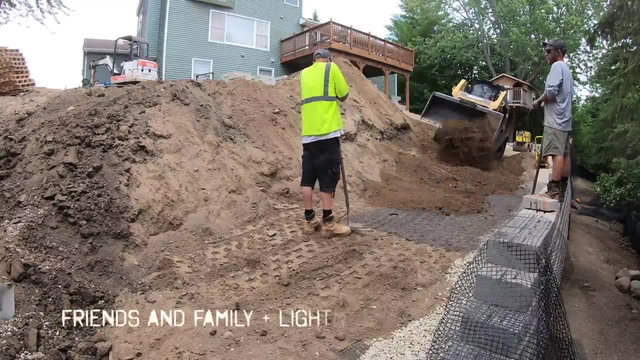 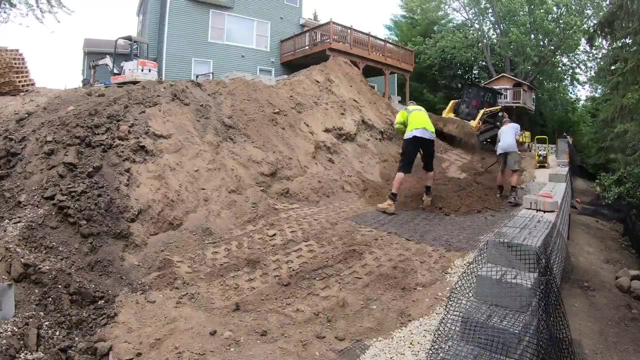 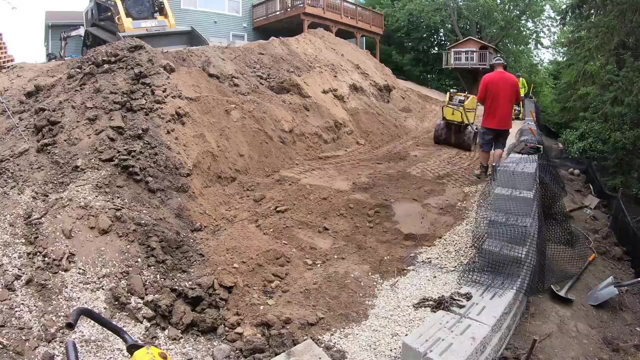 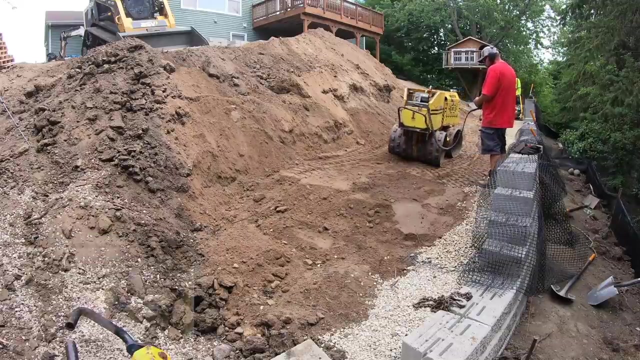 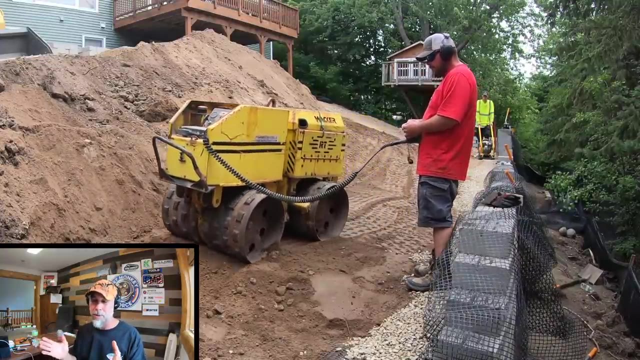 So here he's packing the reinforcements along with our bigger packer. You'll also notice that we typically use the same block on every one of our products, and that's the VersaBlock standard unit, And the reason we use that is simply put. 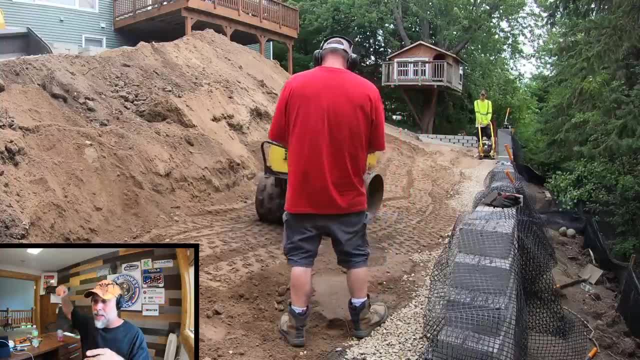 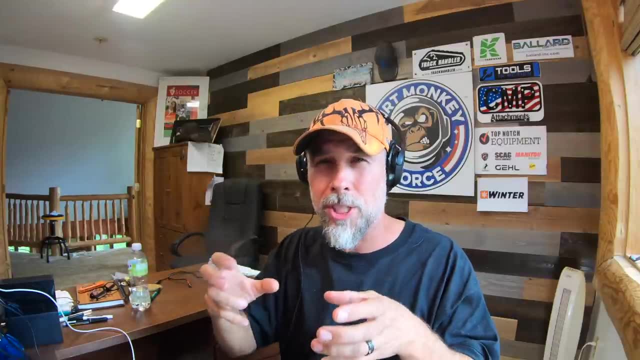 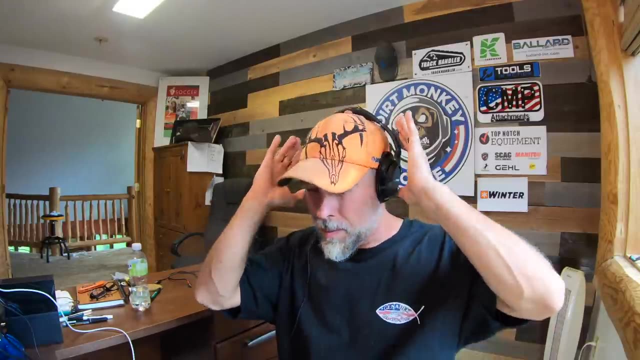 it is the only solid block on the market that is also pinned And that gives us just the confidence, knowing that we're getting a good, solid connection from one block to the next. Now you'll have options with blocks and I want you guys just to kind of put your 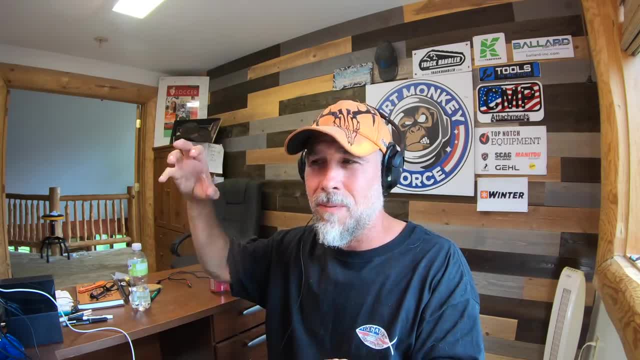 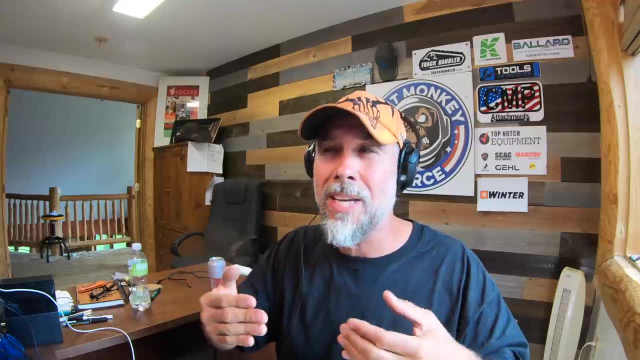 just you know, put your you know, just to put it on your radar screen, to know how blocks actually physically connect together. A lot of blocks don't have pins And what happens is they rely on gravity and weight to stick together. 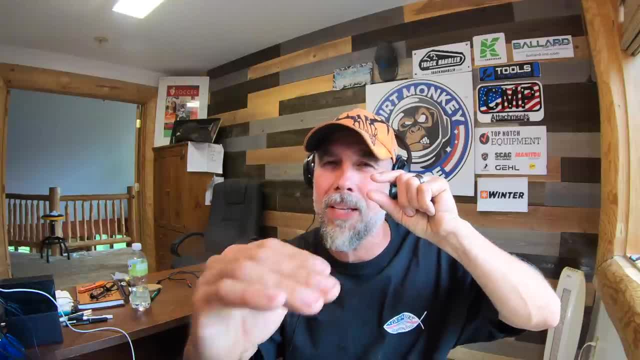 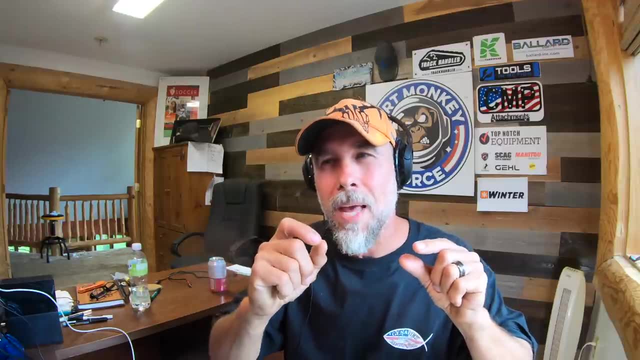 And sometimes they'll have a little tiny lip that runs along the backside of those blocks. You can go to any one of the big box stores and flip a block up and you'll see that little lip. And what that lip does is that lip provides the connection. 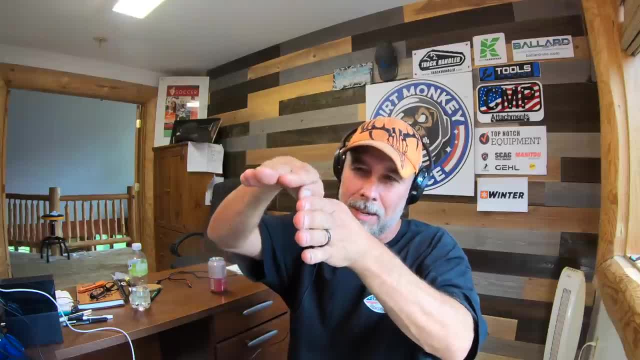 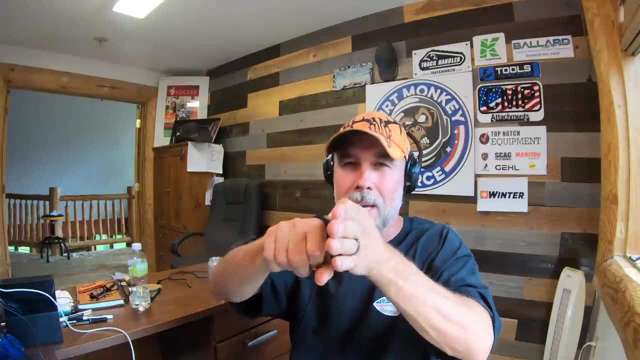 so that the block can't slide up and over. If this is the block and then there's a block underneath it, this block will slide. hit this block, that lip will stop it. But what happens if that lip comes off? There's nothing. 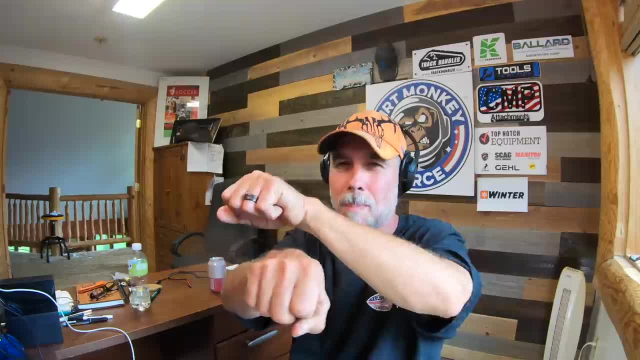 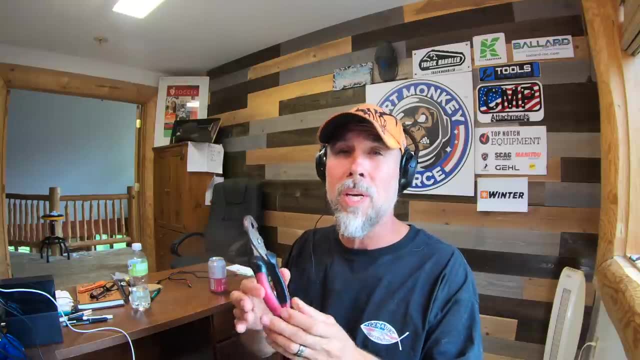 So now these two blocks just are having a slip and slide over the top of each other And those lips do come off. Those lips come off with just nothing much heavier than something like this. We call it a chipping hammer. So when we want to knock that lip off intentionally- 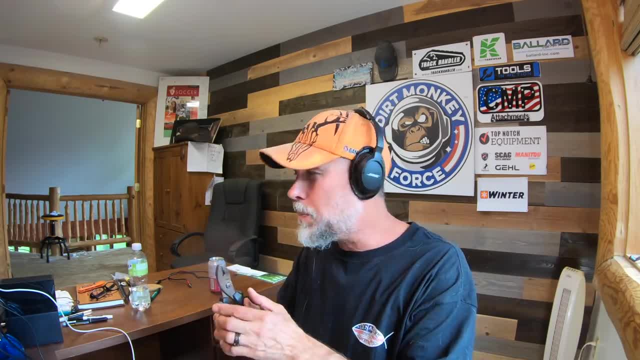 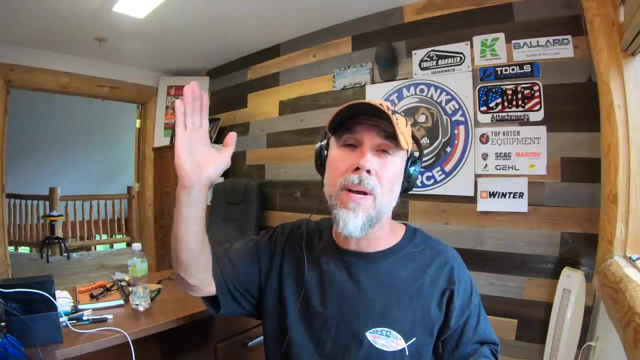 when we got to use those blocks for base. we take a little chipping hammer and we just go: tap, tap, tap, tap, tap, tap, tap along the back of the block And the lip shatters right off And now we've got a flat block on the bottom. 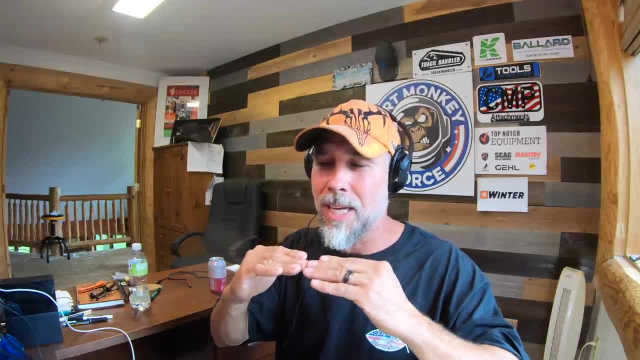 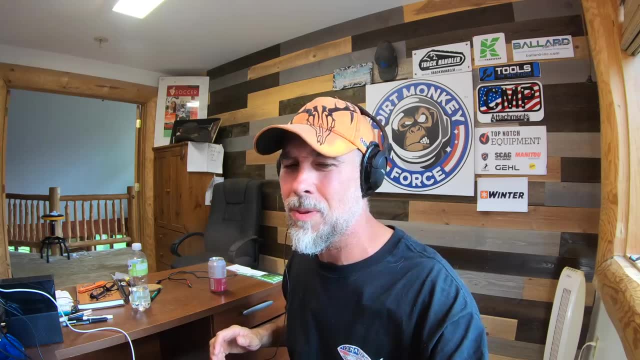 that we can base with. And it was when I came to the realization one day, as I was tapping that back of that block off to base with them, that this might not be the best connection method when I'm starting to build walls that are 9,, 11,, 15,, 25 feet tall. 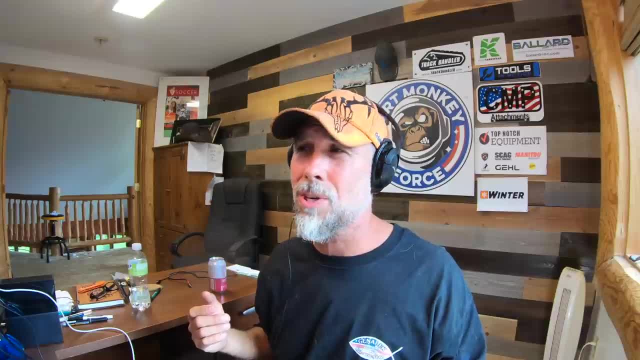 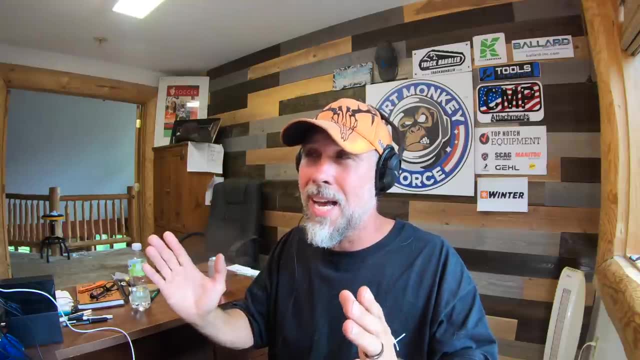 And that's when I started to first use the VersaLock standard units and I've been sold ever since In my book. they have not improved upon the design and I've been using these same blocks for 20-some years. 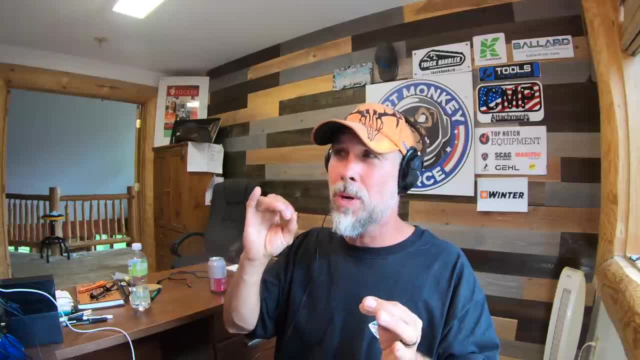 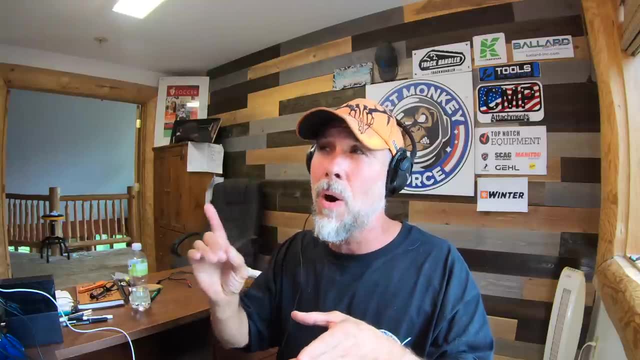 But we've got a lot more video coming down the pipeline. We're going to be tackling a very tricky corner coming up and we're going to wrap this entire project out. And this project actually grows from 9 feet to 11 feet. 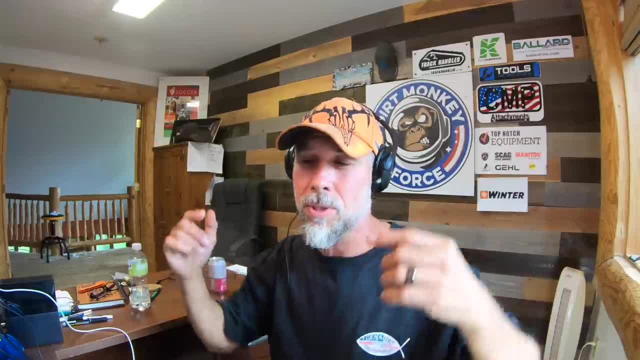 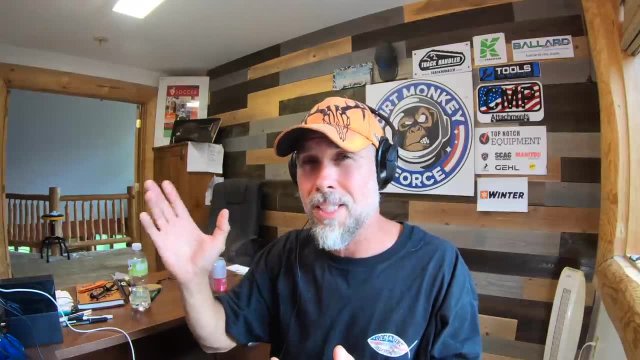 And then we're going to be adding a patio on top of it. So we're also going to have a surcharge placed on top of this retaining wall And this entire wall has actually been designed to actually take. If we wanted to add on to the wall, we could. 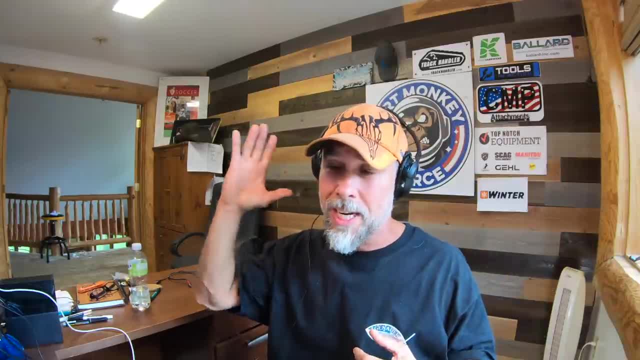 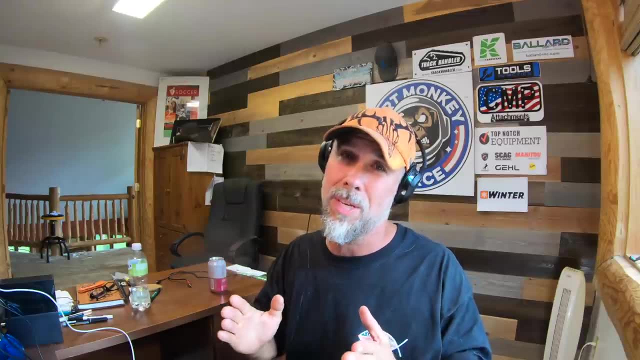 And if we want to place a surcharge on it, we could. We actually designed it ahead of time just in case those two things came up. And on this job site, actually, both of those things came up. They weren't in the initial contract.